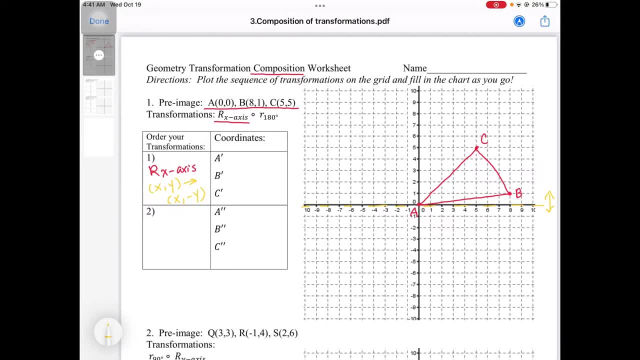 So now I'm going to use this one. So, as you can see, the original is 00. So when I flip that, my coordinates will be 00. My original it's A comma 1.. When I flip that use the formula, it will be A comma negative 1.. 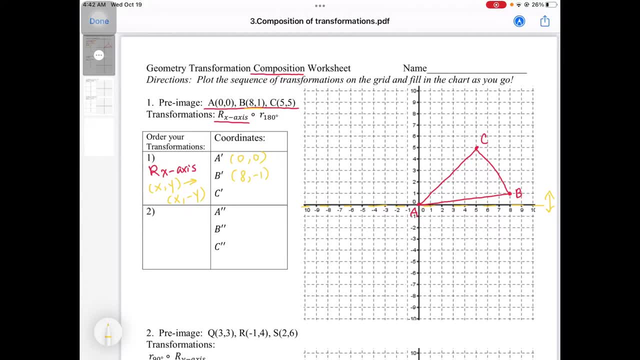 And my original it's 55.. When I flip that over the x-axis that will be 5 comma negative 5.. Or you can say that, Ms Ong, can I just use the shortcut? What do you mean? the shortcut? 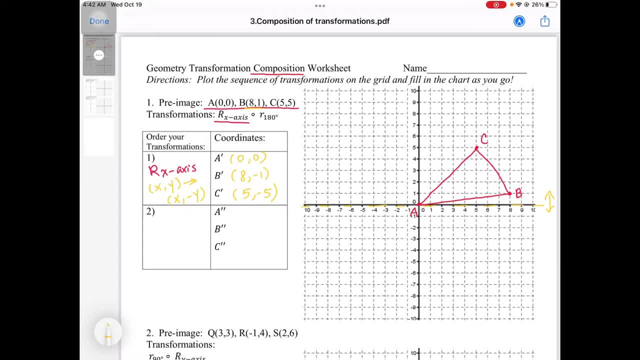 Because with flap they will have the mirror image, They will be the same distance away from the reflection line. So yes, for the B, you will have the same thing over here. So this is my B prime And the C will be 1,, 2,, 3,, 4,, 5.. 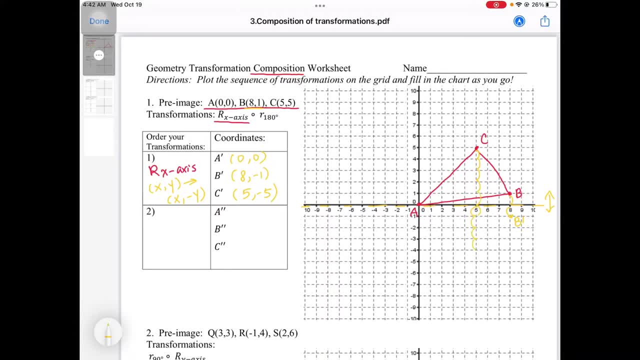 Then you'll be 1,, 2,, 3,, 4,, 5.. So the C it's right here for my C prime And the A it's on my reflection line, So it'll still be my A prime right here. 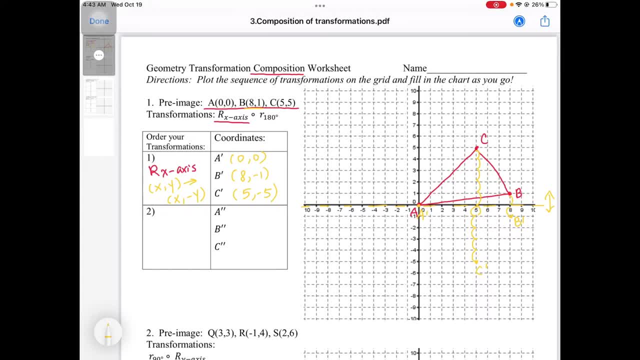 So C is believing. Now you can see your picture of your first transformation, which will be the flip that over the x-axis I'm going to use the dash line to indicate. So my dash line will be here, Right here: Duh, duh, duh, duh, duh, duh, duh. 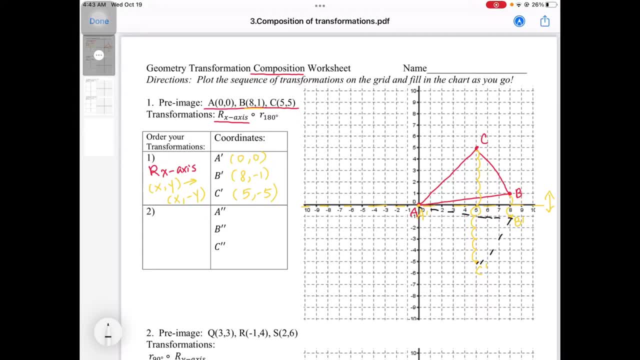 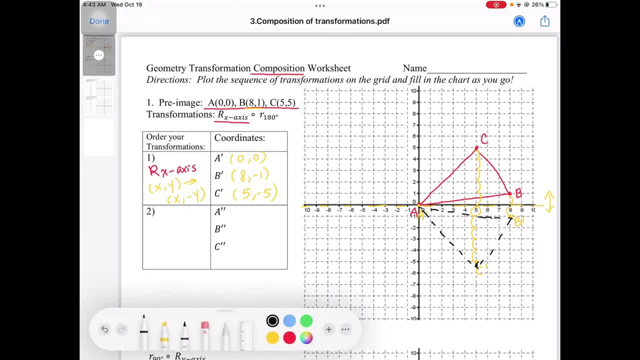 So, moving on to the next one, As you can see here, they want us to rotate. So 180 degrees is a positive. So you know that the rotation is counterclockwise By the formula. we know that the given point. 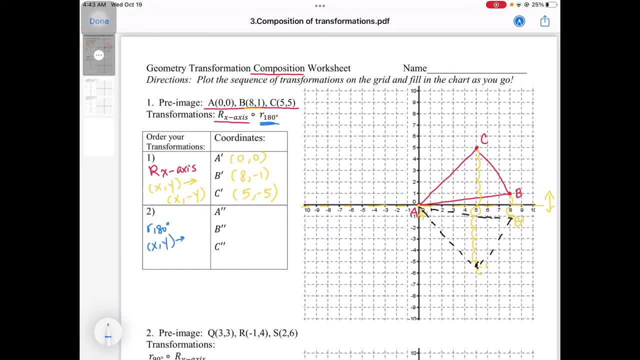 once we rotate 180 degrees, that will be opposite. So negative x, negative y. So again you are coming from your previous step. So we're going to use this point to rotate 180 degrees. So 0, 0, flip that and negative will still be 0, 0. 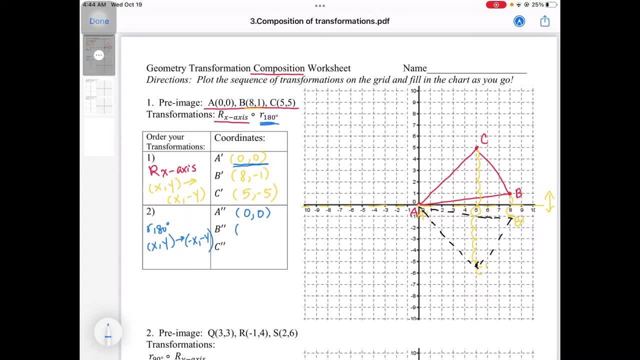 0, 0, right, All right. When I flip that, a negative 1.. So negative, a positive 1.. And when I rotate 180, that becomes negative 5, 5.. So now we can go to the location and plot the new point. 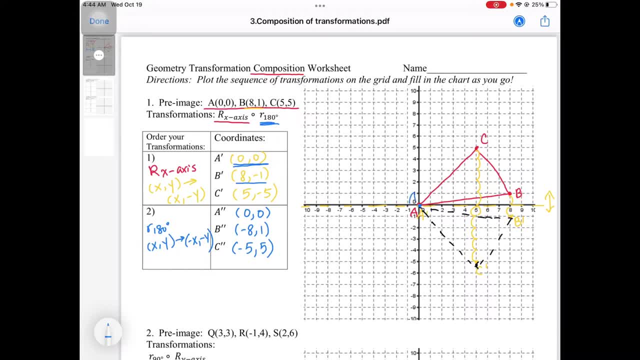 So my a double prime will be right here. This will be my a double prime, And my b double prime will be negative a and 1, which is right here. That will be my b double prime, And my c double prime will be negative 5 and 5,. 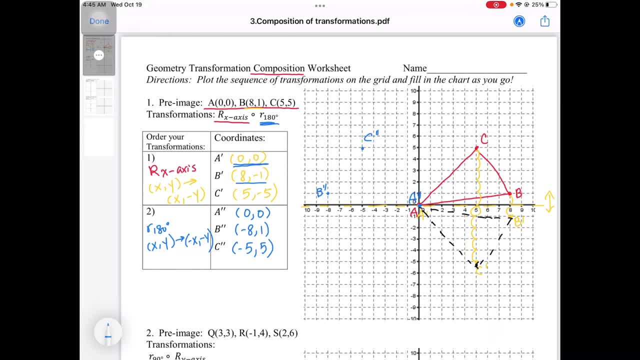 which is right here: c double prime. So we are going to see our final image, which is right here: Ooh la la, Beautifully done. And this is our final image for this transformation After the reflection and the rotation. Good, 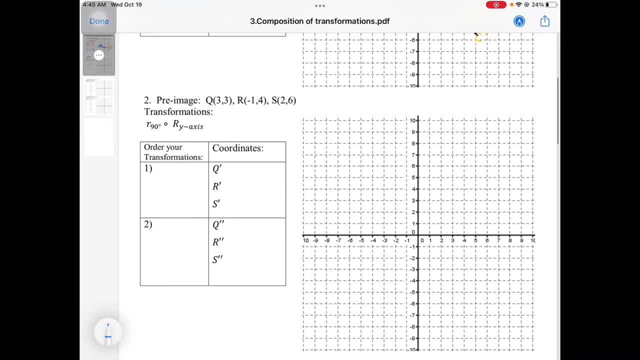 All right, Number two having fun. So we are given this guy preimage. It's located at 3, 3.. So which is right? here? It's my q, 3, 3.. And r it's negative 1 and 4.. 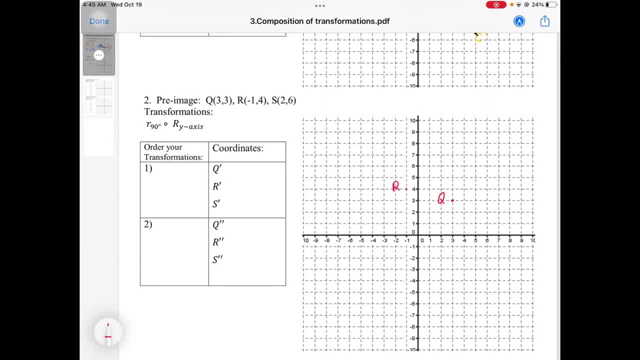 So this is my r And my s is 2, 6.. Which will be my picture? So it's a triangle. So we're going to connect those beautiful points. We get a triangle. All right, What do you want us to have fun with? 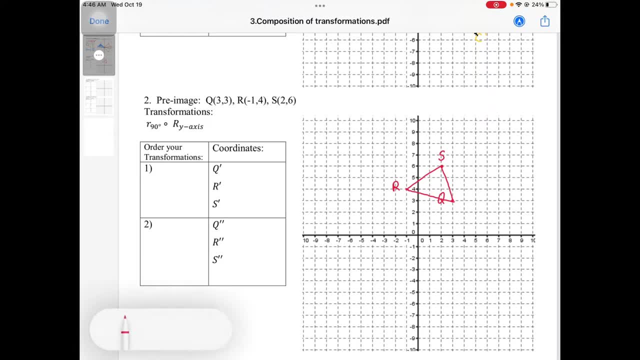 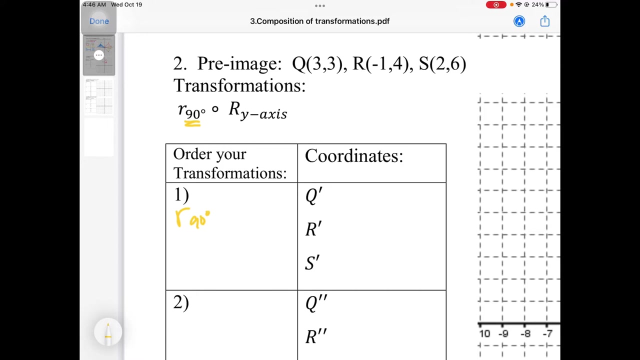 Okay, First they want us to rotate. So when we try to rotate, as you can see here, 90 degree- it's a positive right. So the positive tells us we are going to counterclockwise. So to counterclockwise by your formula. 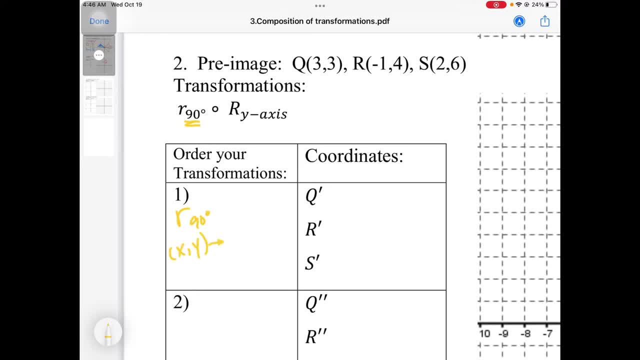 when you're giving the point rotate 90 degree, you are going to flip and put the negative side at the first one. So x and y flip and you're going to put the negative side on the first one. So seeing is believing. 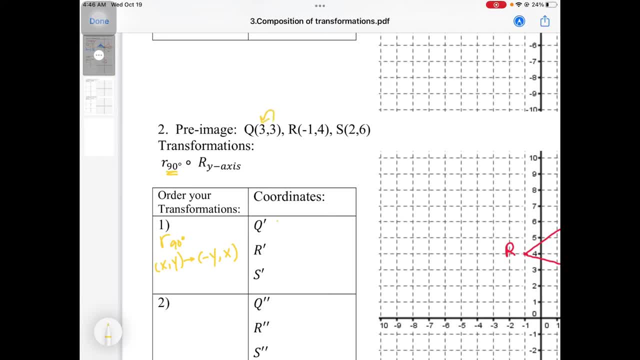 So I'm going to flip and put the negative side on the first one, So that will be negative 3, 3.. I'm going to flip and put the negative side on the first one, So that will be negative 4,, negative 1.. 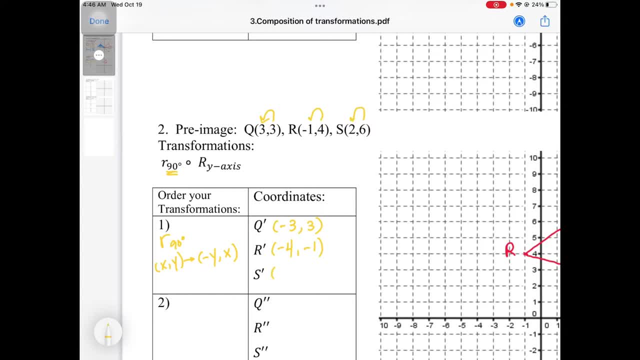 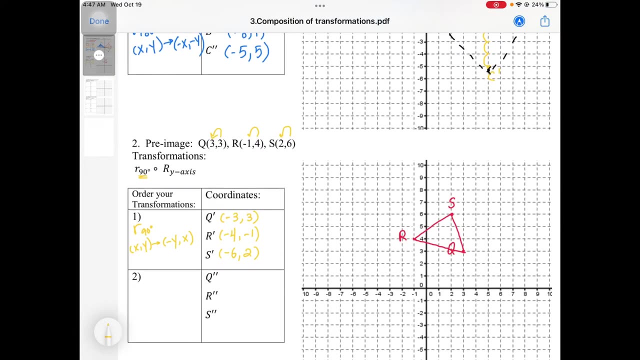 We're going to flip and put the negative side on the first one. So negative 6, 2.. So location, location, location. I am going to plot my transformation for the rotation. So here I: negative 3, 3,, which is right here. 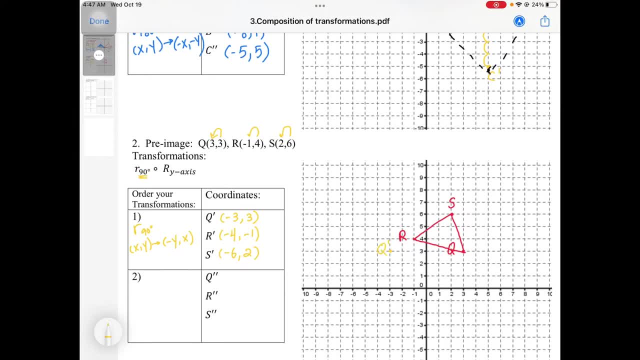 So this will be my Q prime. R prime is negative 4, negative 1,, which is right here. This will be my R prime, And my S prime will be negative 6 and 2,, which is right here. So now you will have your first transformation. 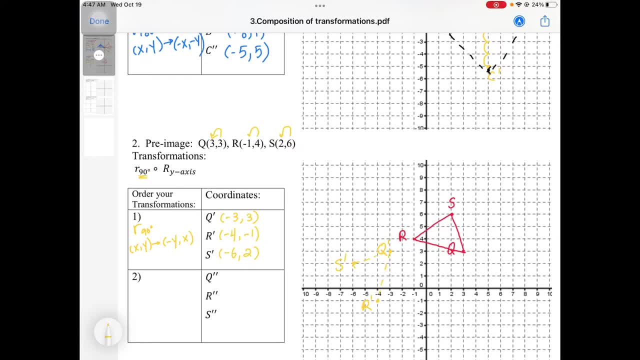 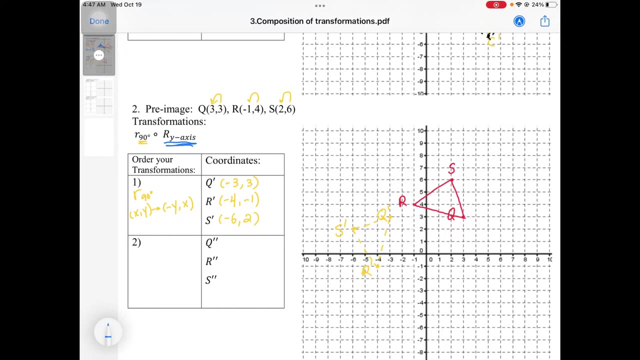 which is right here as our answer, as the picture in dashed line: okay, Moving on, They also want us to reflect, So this time they want us to reflect over the Y axis. So the Y axis, right here, This is the Y axis. 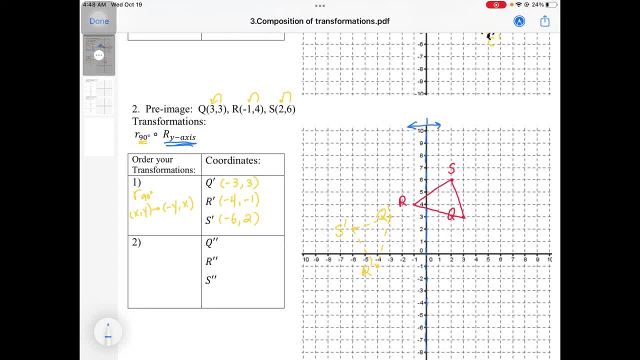 We are going to flip it, which means we're going to left and right. So remember the formula: If we want to reflect across the Y axis, you are going to flip the left and right. So the original is X, comma Y. When you reflect, you are going to left and right switch. 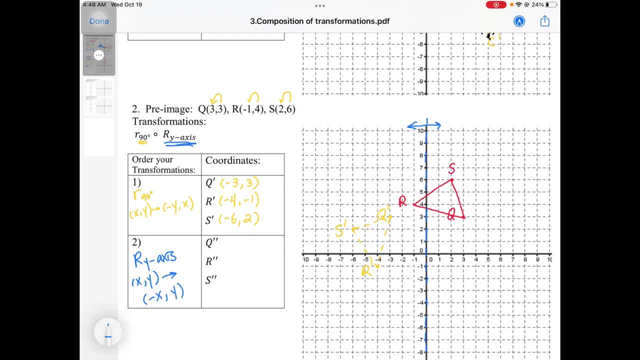 So the X become negative X and Y stays the same. So we are going to flip this guy. We're going to make the X the opposite, So negative 3, negative 3 become a positive 3. But the Y remain the same. 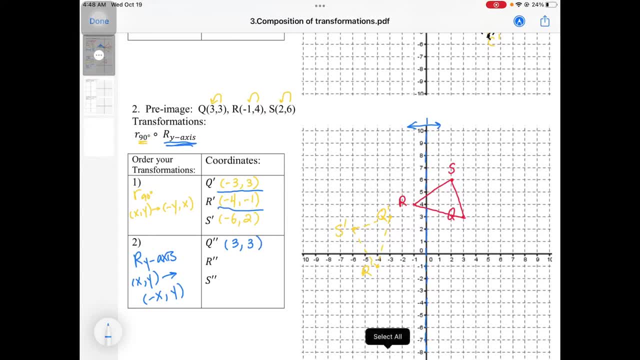 So again, we're going to put the negative sign on X, which will be negative. negative become 4, comma, negative 1 and negative 6, positive, 6 and comma 2.. So now we can say, ooh, I am going to go to the 3,, 3,. 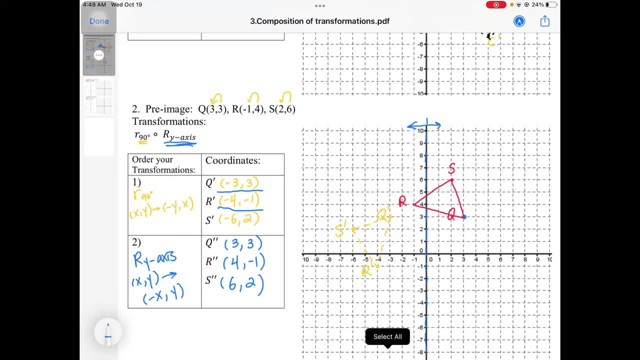 which is right here, That will be my Q double prime And my R double prime will be 4 and negative 1.. Which is right here? It's my R double prime And my S double prime is 6 comma 2,. 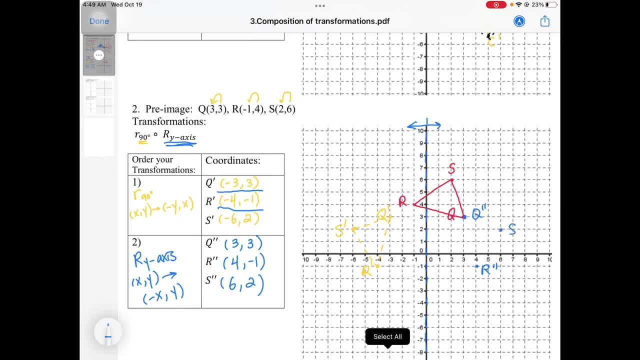 which is right here. That's my S double prime, So connect this picture. You get your perfect answer. Add to your image And it's right here. Now you may say that. Ms Ong, can I still use the shortcut when I do the flip? 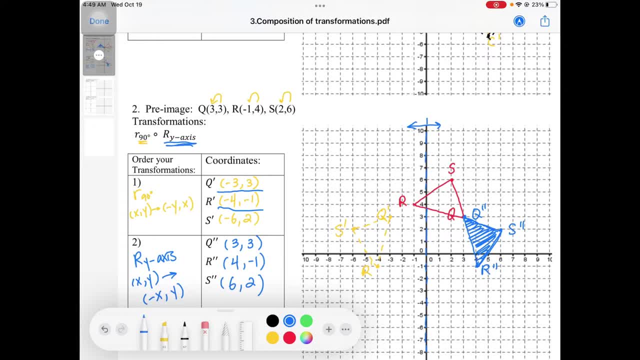 Flip the reflection, Of course. So if you say, how do you know it's correct? Remember the shortcut about the reflection? It is: you have the same distance away from the central light, the reflection light. So if you want to do that, you will see that. 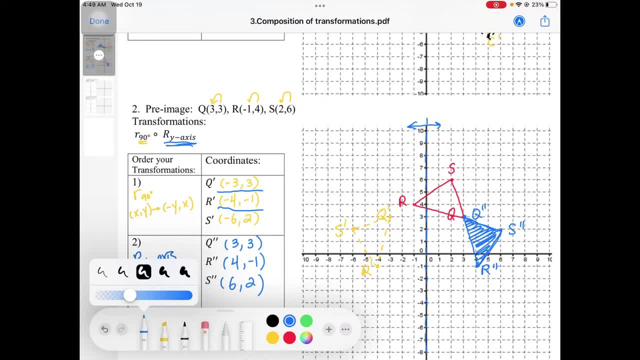 Okay, My original, my original Q prime. it is 1,, 2, 3 away from the reflection line, So I'm going to flip that to the right side will be 1,, 2,, 3.. And my original S prime: 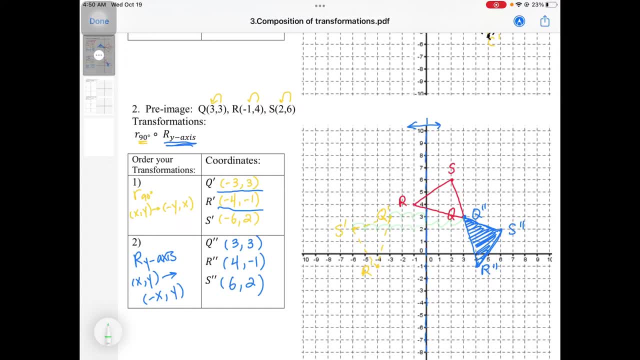 it's 1,, 2,, 3,, 4,, 5, 6 away from the reflection line, So from left, I'm going to flip that to the right, So that will be 1,, 2,, 3,, 4,, 5, 6.. 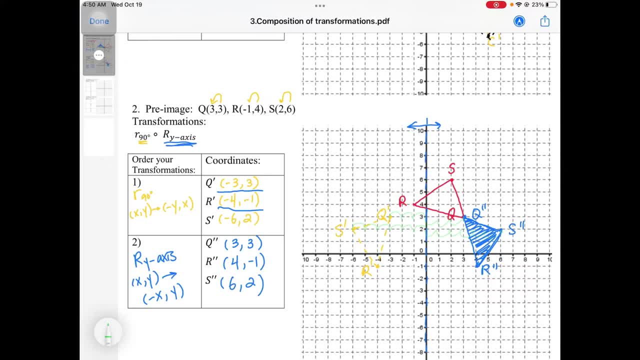 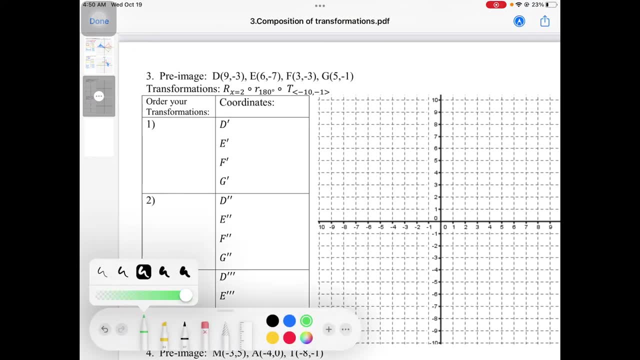 So we will get the same distance. Okay, So you're welcome to use the shortcut as well. Okie, dokie, Number three: given the pre image, as you can see here, it's D, E, F, G, So let's go. 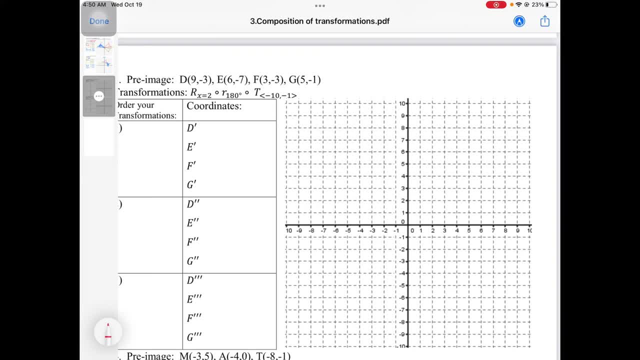 9, negative 3.. So 9, negative 3.. It's right here, That's my D And E is 6, negative 7.. 6, negative 7 is right here, It's my E And my F is 3, negative 3,. 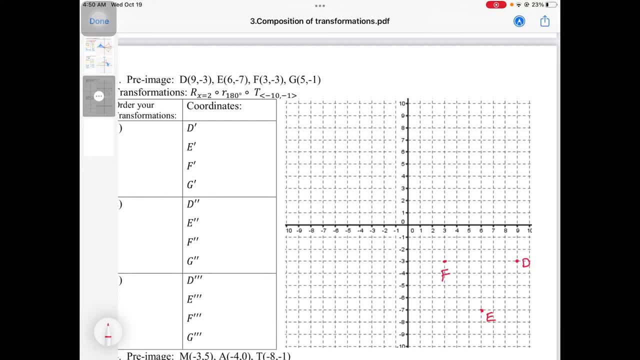 which will be right here, And my G is 5, negative 1, which is right here. So seeing is believing. We have a quadrilateral. We have a four side picture, Right, Maybe you will say it will be a trapezoid. 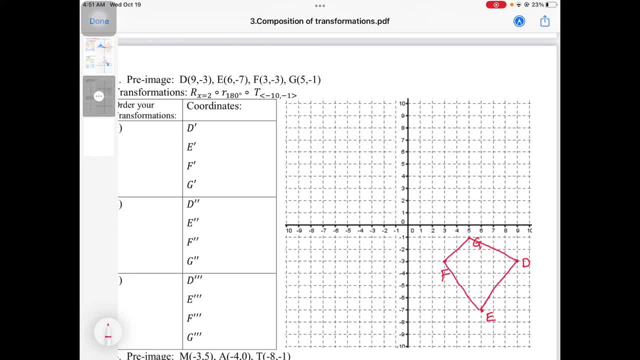 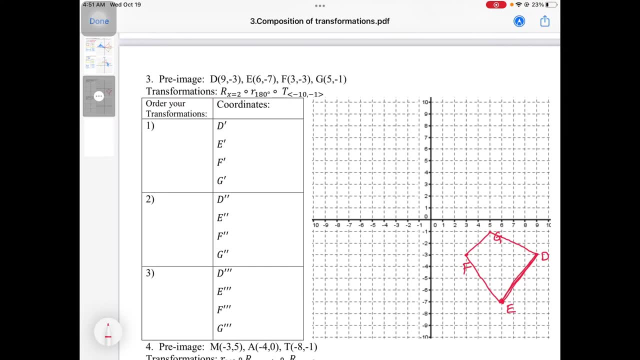 Looks like that: right, Two parallel set. All right, This is our pre image. So now they would like us to do some transformation. Let's see what's going on. So first one: they want us to reflect over the X equal to 2.. 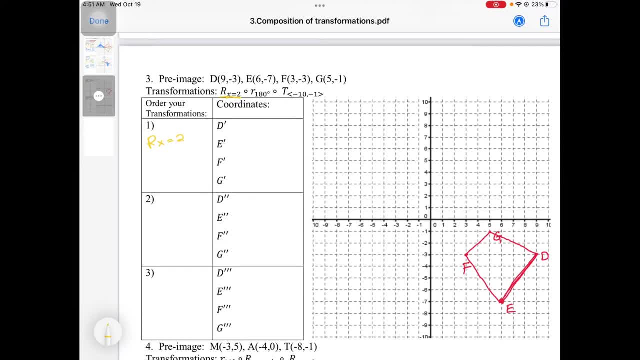 So the X equal to 2,. step one: reflection. we are going to locate the reflection line So X equal to 2, which is right here. So this is our reflection line: X equal to 2.. This is equal to 2.. 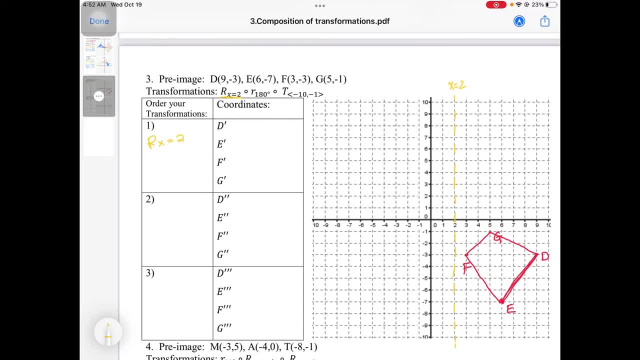 X equal to 2.. So you know that this reflect- we're going to have a flip, It's a left over right, This switch. So by the formula, by the formula, you know that we can use the coordinate or you can say zone. 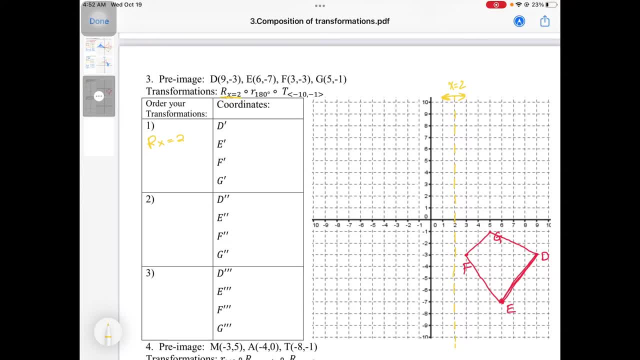 We can just use the shortcut. So, yes, indeed, So we know that if you using the same distance away from the central line, which will be the reflection line, So the F will be flipped to the left side from right, So it's one unit. 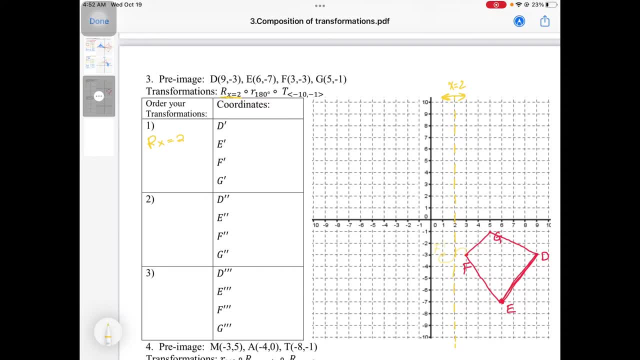 So that will be my F prime. So that will be my F prime. I'm going to use this one. So F is one unit. Now I flip to the other side, So F prime is right here. Right here is my F prime. 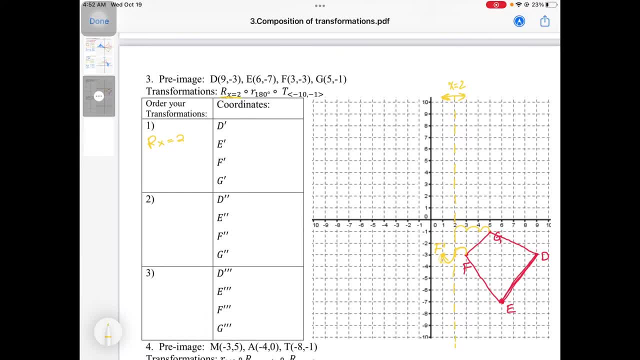 And G will be 1, 2, 3.. So that will be 1, 2, 3.. So G prime is right here And D 1,, 2,, 3,, 4,, 5.. 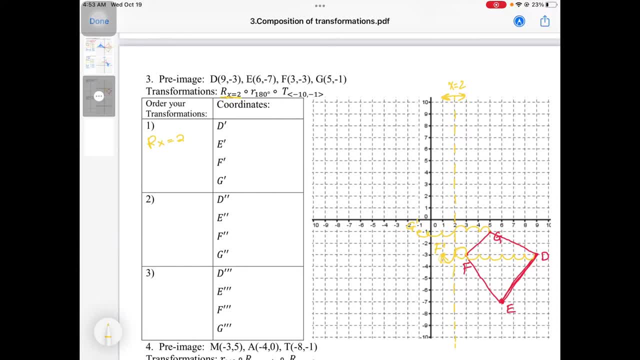 1, 2,, 3,, 4,, 5,, 6, 7.. So now we need to flip to the other side: 1, 2,, 3,, 4,, 5,, 6,, 7.. 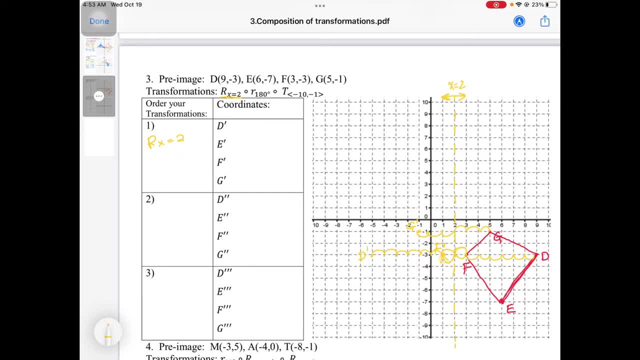 And this will be my D prime And E. that will be 1,, 2,, 3,, 4.. So flip to the other side: 1,, 2,, 3,, 4.. So I have my E prime. 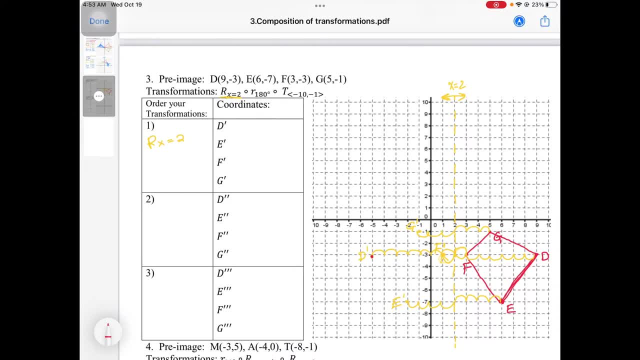 So use your ego at this moment. okay, D is right here, D prime is right here, G prime is right here, F prime is right here And E prime is right here. So now can you tell me what you see is what you got? 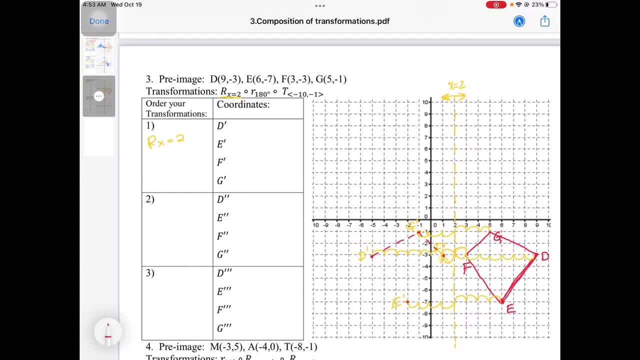 Do you see your coordinate of my new shape when I reflect over the X equal to 2?? Yes, So ego at D prime, It's believing D prime. we got negative 5 and negative 3.. So negative 5 and negative 3.. 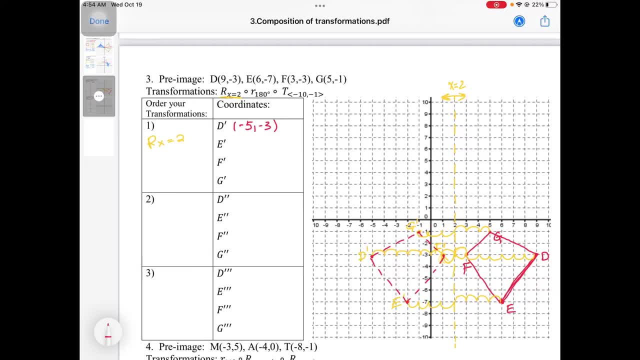 And E prime. it's negative, 2, negative, 7.. So negative, 2, negative, 7.. C is believing And my F prime- right here is my F prime, It's 1, negative, 3.. 1, negative 3.. 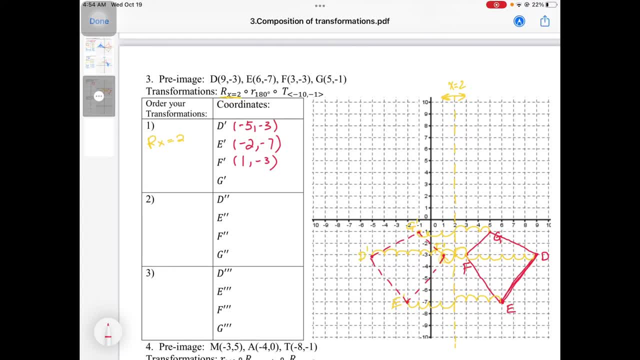 My F prime, it's 1, negative 3.. And my G prime, as you can see here, is negative 1, negative 1.. So negative 1, negative 1.. So again, when there is a picture, the answer is in the picture, okay. 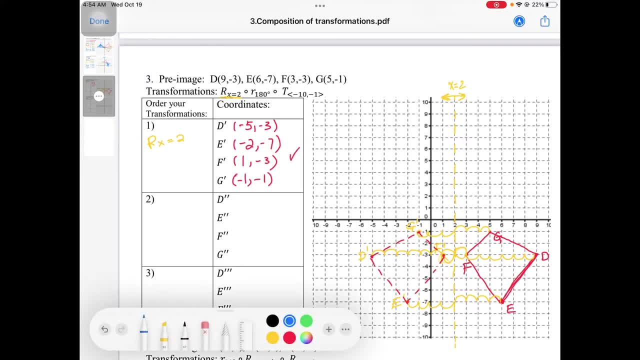 So now we can move on. The next one they want us to do is to rotate 180 degree. So we are going to rotate 180 degree. again, It's a positive, so you know that it will rotate counterclockwise. So by the formula you know that the rotation about 180 degree you are going to negative, both. 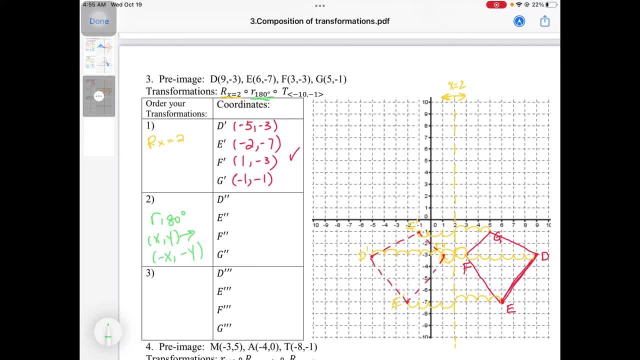 So you will have negative X and negative Y. So we are going to put a negative sign from the previous step. So my D double prime, which will be 5, 3.. And my E double prime will be 2, 7.. 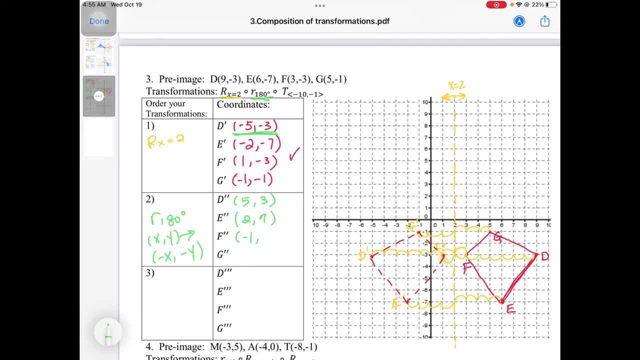 And my F double prime will be negative 1 and positive 3.. And my G double prime will be 1,, 1.. So location, location, location. So 5, 3.. So 5, 3, it's right here. 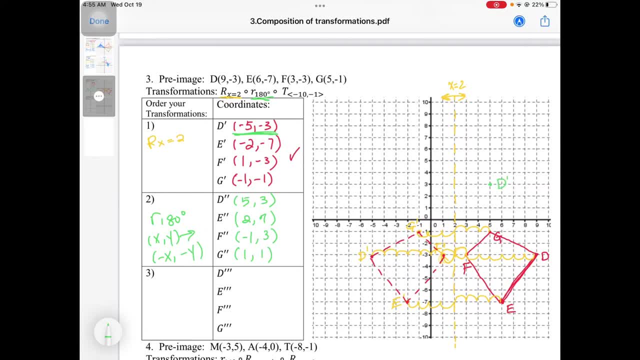 So this is my D double prime And I have 2, 7.. 2, 7,, which is right here, That is my E double prime. I got F double prime. it's a negative 1 and 3.. 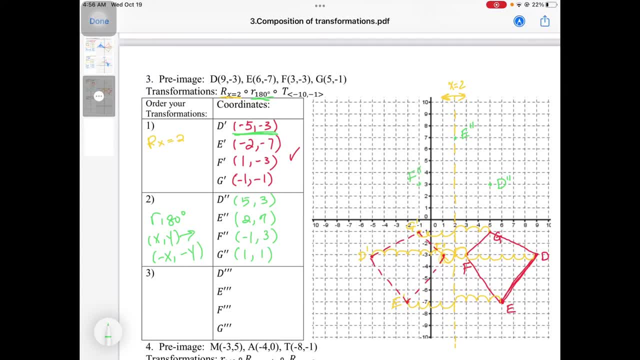 So this is my F double prime And my G double prime. it's at 1, 1.. This is my G double prime, So C is believing. Now my picture: it's rotate 180 degree, Counterclockwise. 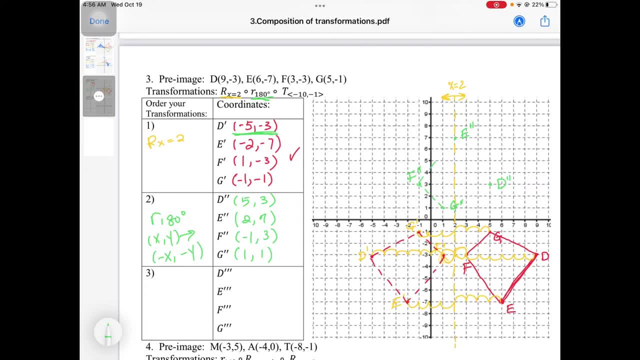 And it come to this location. And this is my picture. Beautifully done. Okay, Alright, very last one, The last one. they want us to do a translation slide. So C is believing, So you know that the translation. they want us to have the X. 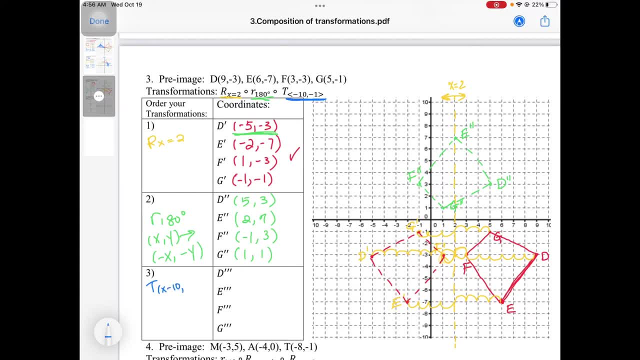 We're going to moving down 10 units. And the Y you're going to moving down. I'm saying this wrong thing. The X minus 10 means you're going to the left. So you're going to left 10 and down 1.. 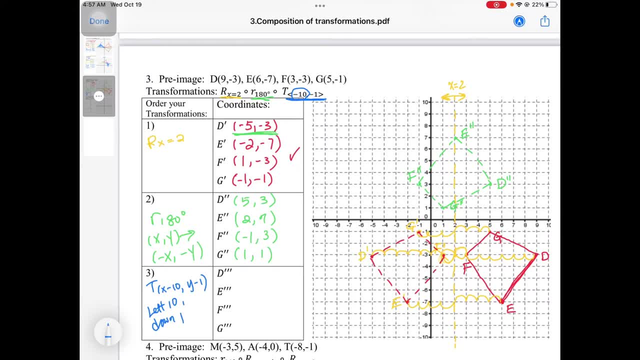 So here we go, Which tells us: you can use the shortcut or you can use the algebraic. So left 10, which means 5 need to minus 10.. And 3 need to minus 1.. So 5 minus 10, which become negative 5.. 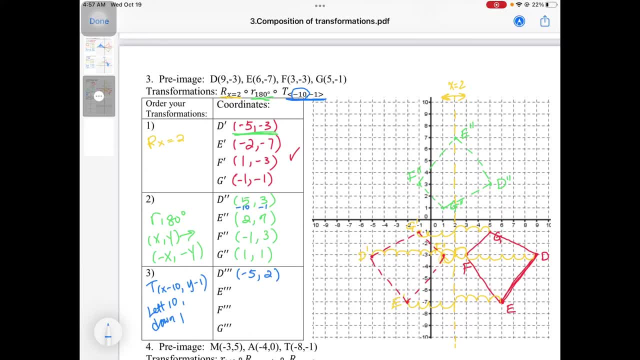 And 3 minus 1, which become 2. So we can still get that. So following: So: 2 minus 5 will be negative 3. And 7 minus 1 will be 6. And negative 1 minus 10, it become negative 11.. 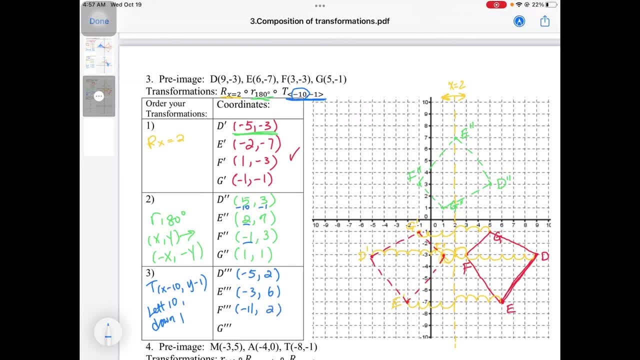 And 3 minus 1 become 2.. And next one: 1 minus 10. That will be negative 9. And 1 minus 1. That will be 0. So this is our correct answer, right? So location, location. 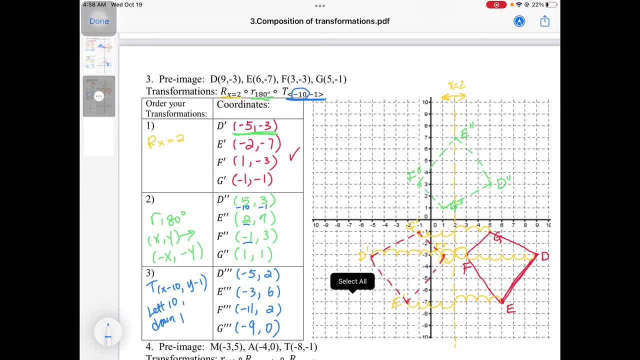 D triple prime. So negative 5 and 2, which will be right here. So this will be my D triple prime. Or you can say: Can I just use my movement Down 10.. Sorry, Sorry, Left 10 and down 1.. 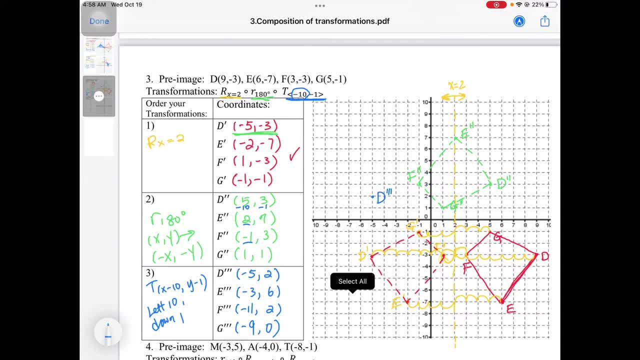 Yes, Let's take a look at that. Do I do something wrong? Negative: 5 and 2.. And then, And then we're going to do this one, Okay, So D movement, Okay, Nope. So now what will be my next one? 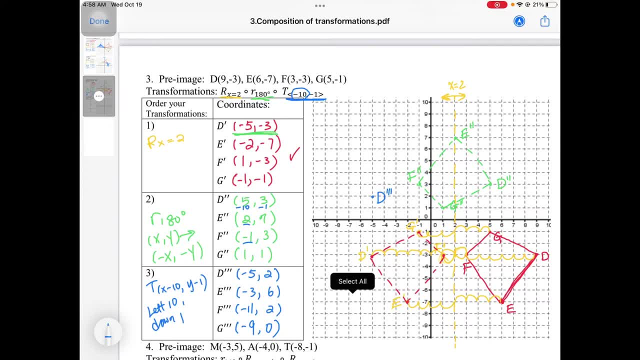 Which will be negative 3, 6.. Negative 3, 6. Which will be right here: Negative 3, 6. That will be my E triple prime And I have an F triple prime. Negative 11, 2.. 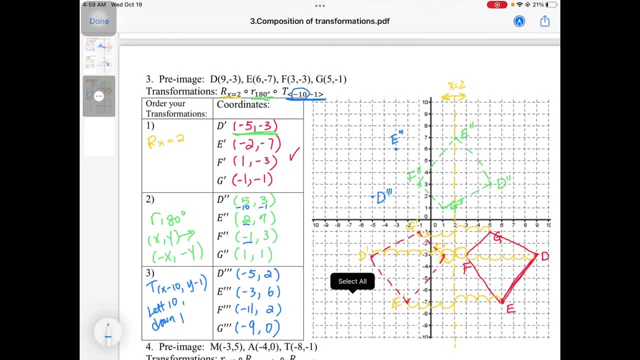 Whoa All the way out, But it's okay. Negative: 11 and 2.. So, which will be right here? That will be my F triple prime And G triple prime. negative: 9, 0.. Which will be right here. 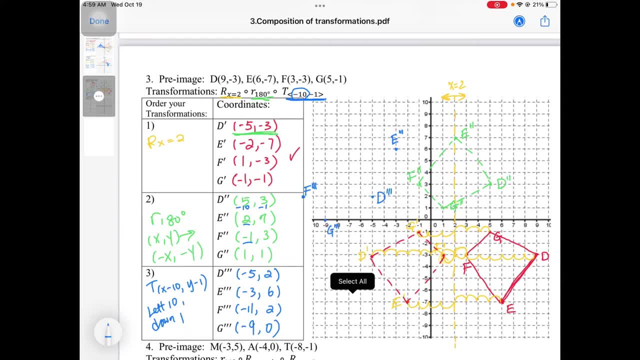 This will be my G. So now, if you say, Ms Hong, What's going on about? my final answer, Why I see something is different. Do I make a mistake? Let's check. I have a. Oh, You know what I make a mistake here. 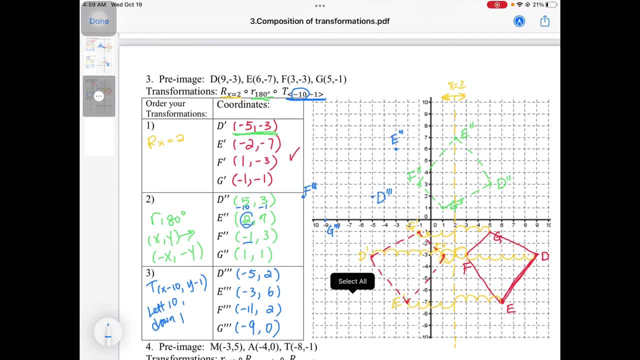 2 minus 10.. 2 minus 10.. That should be what Negative 8.. Wow, Glad we have our eagle eye, So I have a mistake right here. The E double prime. How do I know that? Because picture look different. 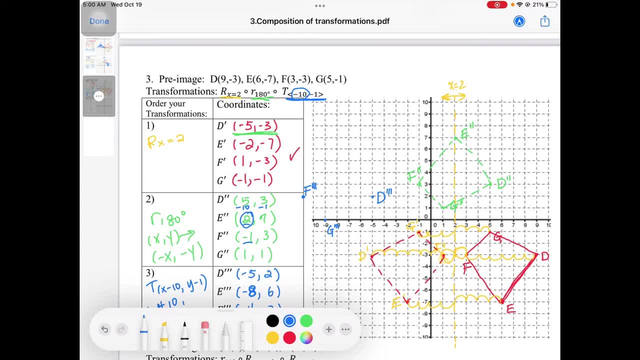 So I know that: Negative 8 and 6. Negative 8 and 6. Which is right here. So now I have This is my E triple prime, So now I have a better picture about that, So my picture will be right here. 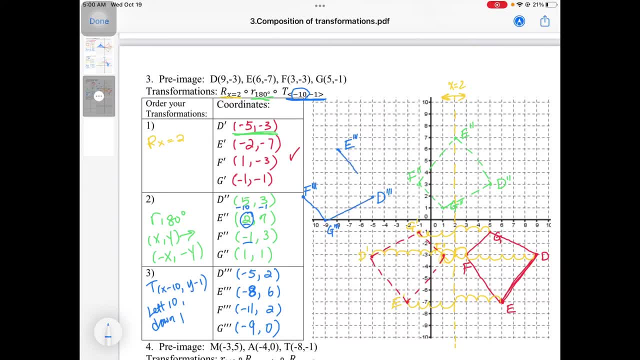 Connect the point Much better. So this will be my final answer For this transformation. Now, If you say, Ms Hong, You said that we can use the shortcut right When we slide. Yes, So let's check that. 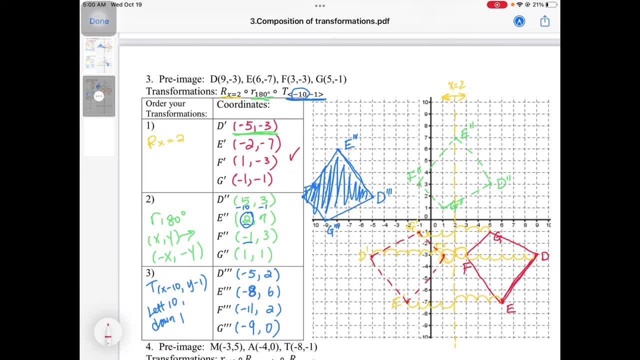 So F double prime. It's right here When you try to Move 10 to the left. So we're going to move 1., 1., 2., 3., 4., 5., 6.. 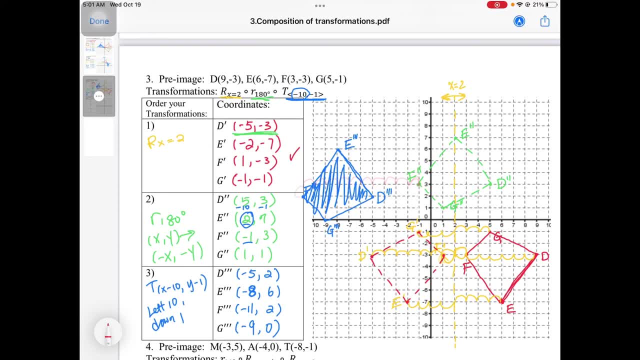 7., 8., 9., 10.. You're going to move down one, So this is the right correction. You are in right here. Check: Same thing as the E. You're going to move to the left 10 units. 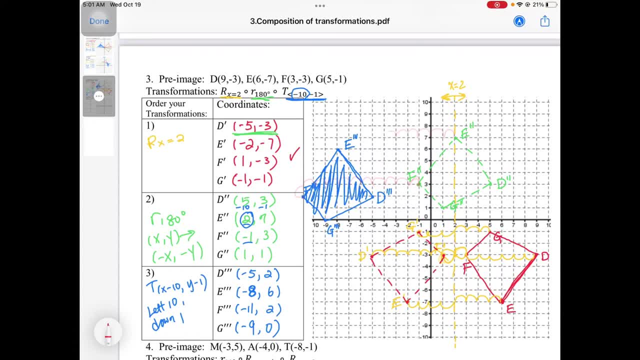 1., 2., 3., 4., 5., 6., 7., 8., 9., 10. And you need to move down, So this will be the down, And we are at the same location as well. 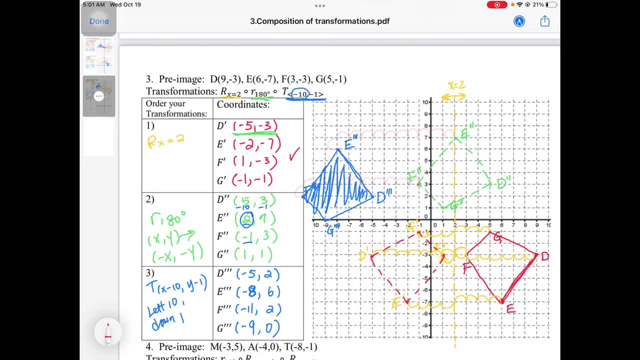 So this is the fun thing about Using the picture: Use your ego eye, Okay. Last one, We have a pre image Given to us. It's a triangle again. So the M, It's negative 3 and 5.. 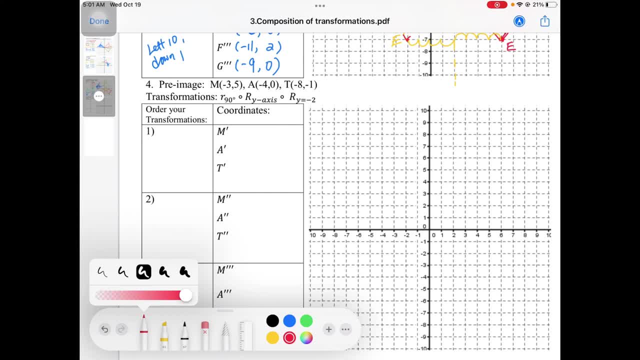 So negative. 3 and 5.. It's right here That It's my M And we get A. It's negative 4.. 0. Which is right here, A We get T. It's negative 8.. 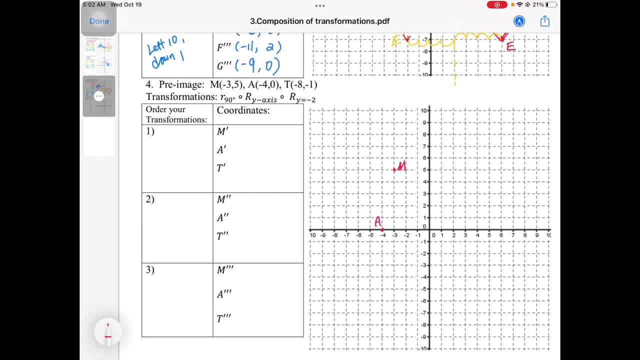 And negative 1.. So That It's negative 4.. 0.. Which is right here. A It's negative 1.. So This It's my T Picture. See It's believing We get. 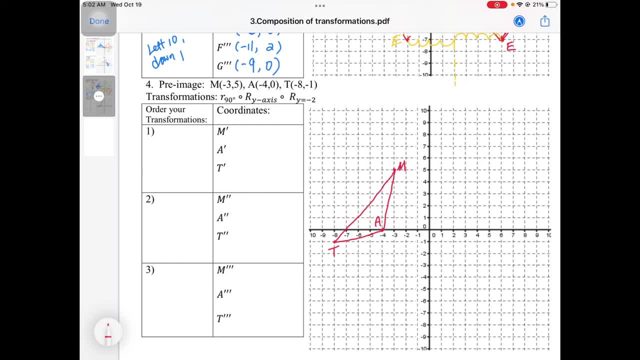 A triangle Right here, Perfect. So Now We are going to perform. We have A Rotation 90 degree, So The rotation 90 degree, Again It's a positive degree. So We know that. 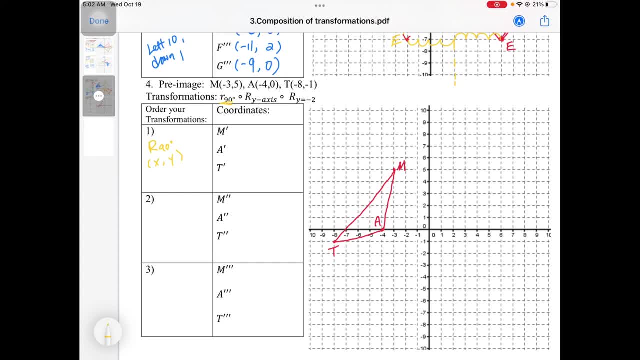 It will rotate Counterclockwise. You're going to turn to the right. Okay, So We are going to flip The x and y And put the negative side On the first one. So I get to flip it. 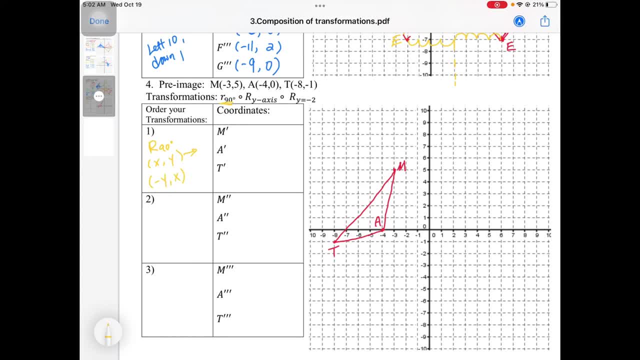 So I get to flip it. So It will be Negative 5.. Come on Negative 3.. Check, We're going to flip it. So That will be 0.. Come on Negative 4. Now. 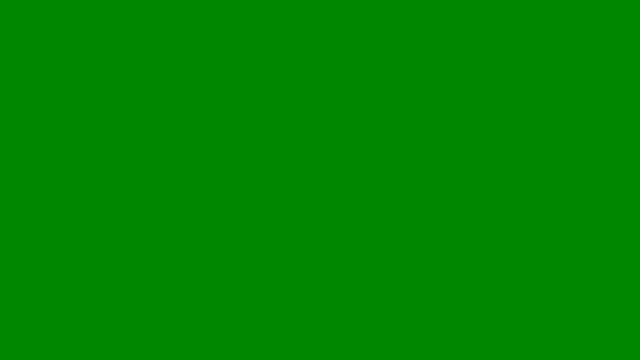 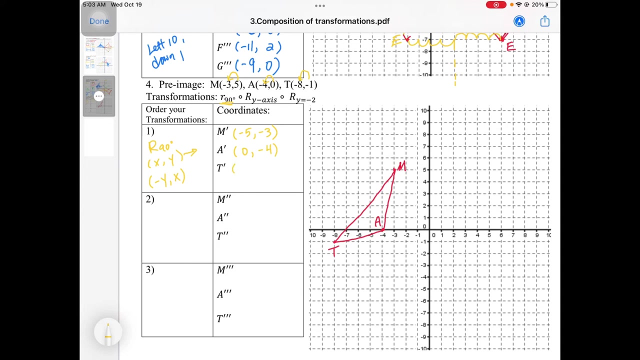 Negative 0.. Still be 0.. Okay, We're going to flip it So Negative 1. We're going to Put the negative side On the first one. So Negative, Negative Become Positive. So 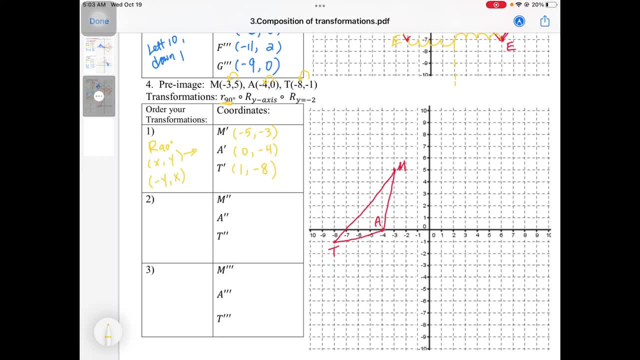 That will be Positive 1. And Negative 8. This is correct, So Let's go. Negative 5. And Negative 3.. So This will be My 8 prime: 0. Negative 4.. 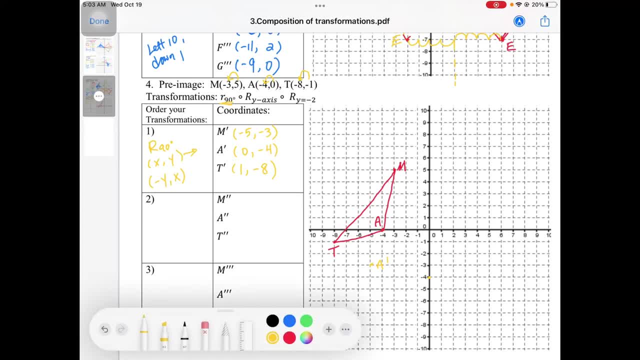 0. Negative 4. It's right here. That is My 8 prime. You got Negative 5. Negative 3.. This is My M prime, And 0. Negative 4. That is. 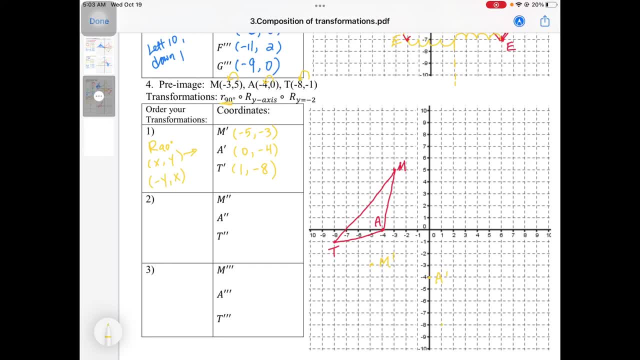 My 8 prime And 1. Negative 8.. 1. Negative 8. That is My T prime. So We do Have Our Triangle After My Home All. 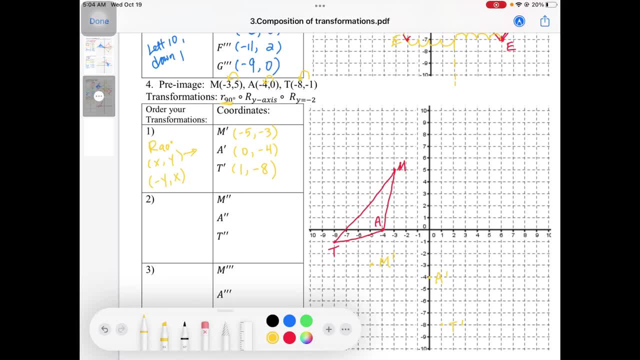 Right Be Professional, Draw The Picture Nicely, So Connect The Dot. Connect The Dot Better This Time. Okay, So Now Step 2. They Want Us. 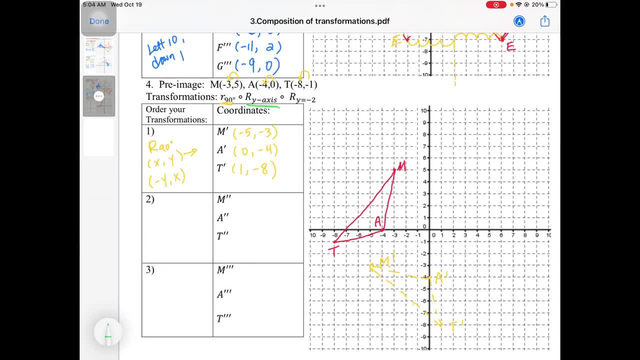 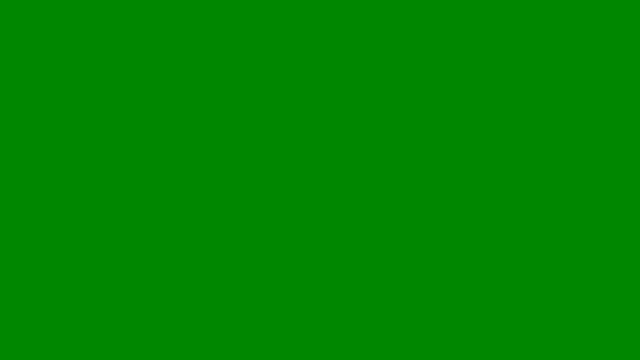 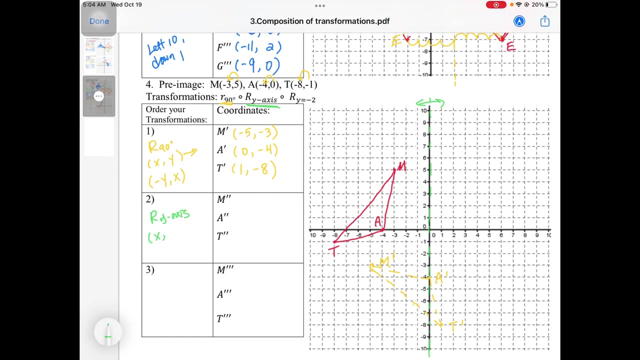 To Reflect. So Step 1. You Can Always Locate Your Reflection Line. So This Time Is The Y Axis. So We Know That The Y 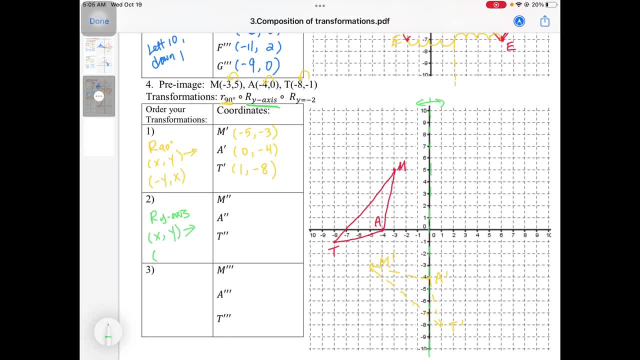 Axis You Are Going To Flip, So We're Going To Use The Previous One. So That Will Become Negative, Negative Five, Become Positive Five And 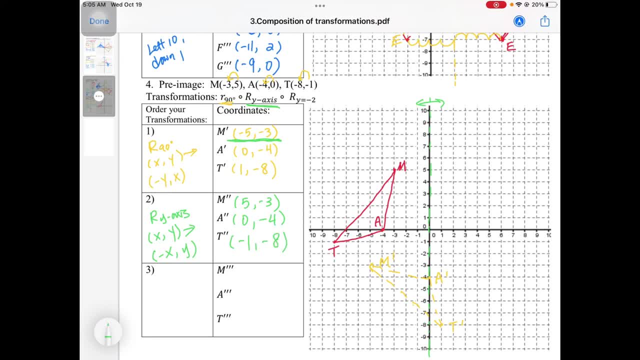 Negative Three And The A Prime Will Be Zero Come Negative Four. So Still Be Right Here, That Still Be My A Double Prime And My. 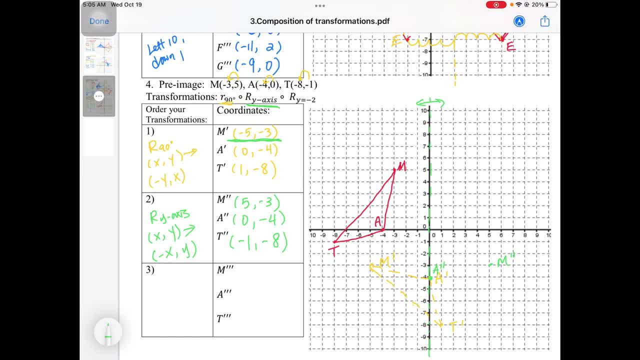 T Double Prime Will Be Negative One, Negative A, Which Is Right Here T Here Nice. So The Triangle Flip Left To Right. Okay, What We? 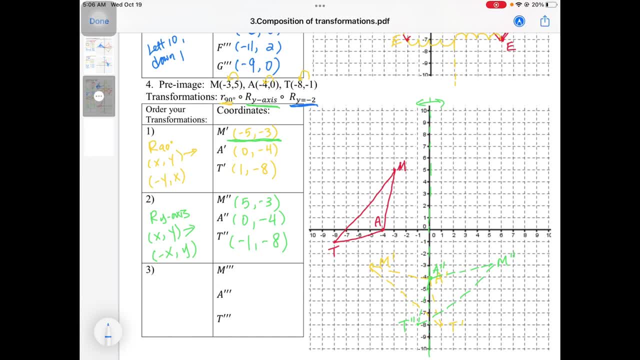 Need To Do As The Very Last Transformation. Oh, They Want Us To, So We Going To Have A Flip. So Again, This Moment I'm 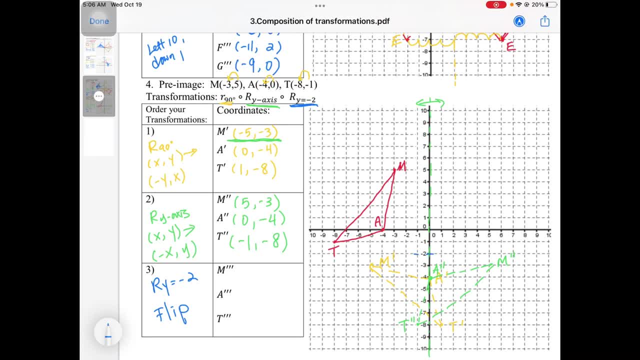 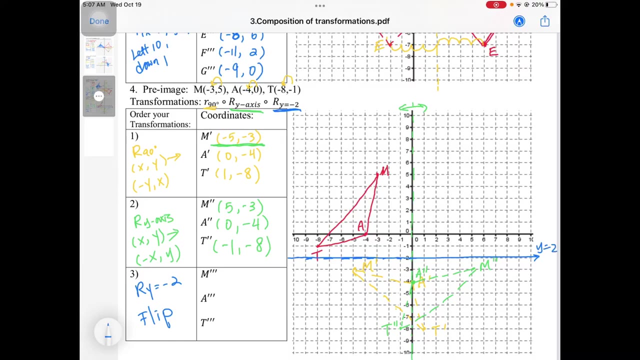 Going To Use The Stroke Up, Excuse Me So Location, Location, Location Y Equal To Negative. My Y Equal To Negative. To Y Equal To. 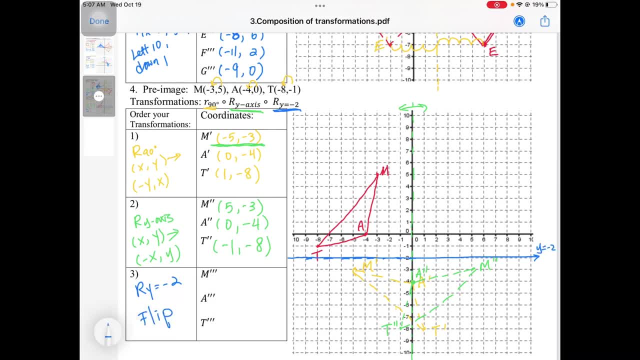 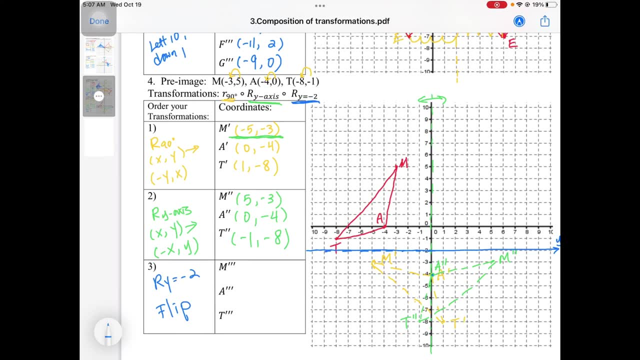 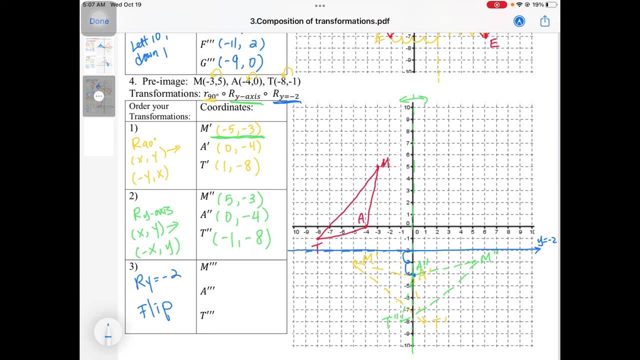 Negative To. So, As You Can See Here, You Are Going To Have A Flip Which Will Be Upside Down. That's My A Triple Pride.